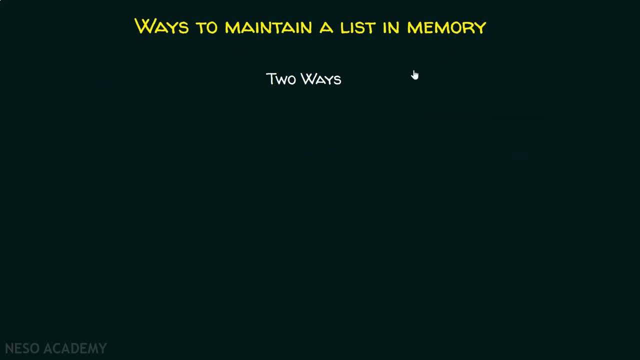 In order to maintain a list in a memory, there are basically two ways available with us. The first one is, of course, by using a list Using array data structure. The other one is using link list data structure. By using these two ways, we can maintain a list in a memory. 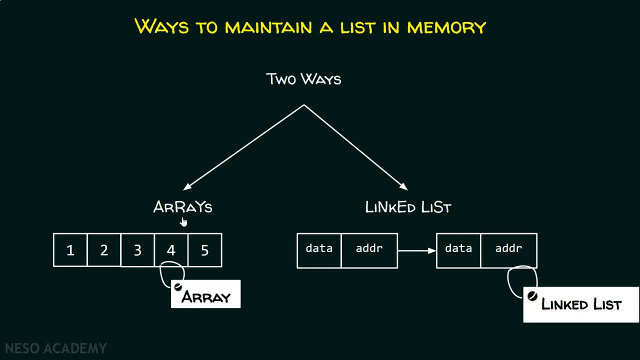 These are basically the data structures. We have already dealt with array data structure. Now in this presentation and in the subsequent presentation, we will deal with how to maintain a list using link list. Arrays have some limitations and disadvantages, and there is no doubt about it. 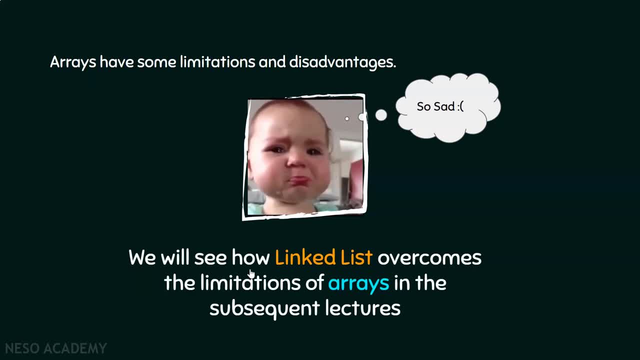 This is very sad, But we will see how link list overcomes the limitations and disadvantages of arrays. We will see what are the disadvantages and limitations of arrays And we will see how link list overcomes those limitations and disadvantages in the subsequent lectures. 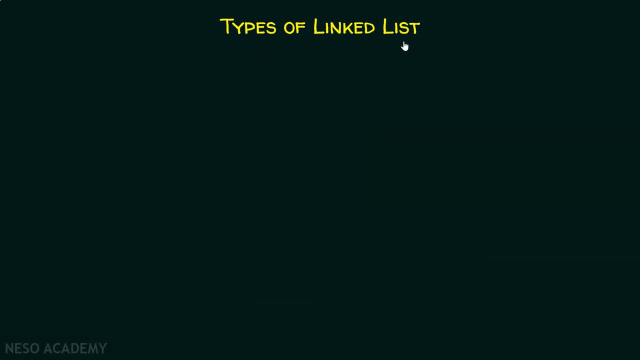 But for now we will see what are the different types of link list we are available with. The first one is, of course, single link list. This is the basic type and the first type of link list. Basically, in single link list, navigation is forward only. 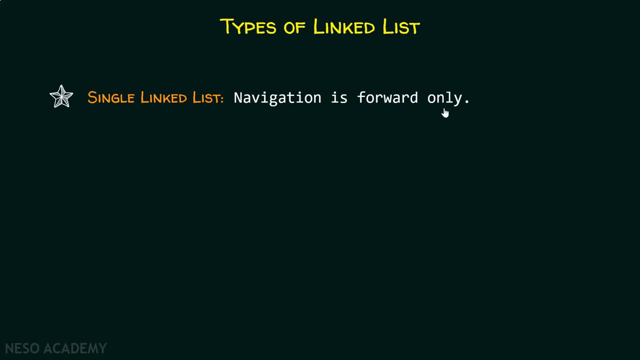 That means we can go in forward direction and we can't go backwards. So navigation is forward only This is the way we can identify a link list as a single link list. When the navigation is forward, only then it is called as a single link list. 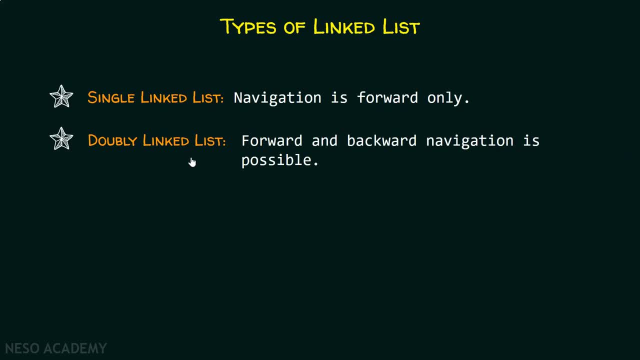 But when the navigation is forward and backward then it is called a doubly link list. So here in the doubly link list forward and backward navigation is possible. We have another type, called circular link list. Here the last element is linked to the first element. 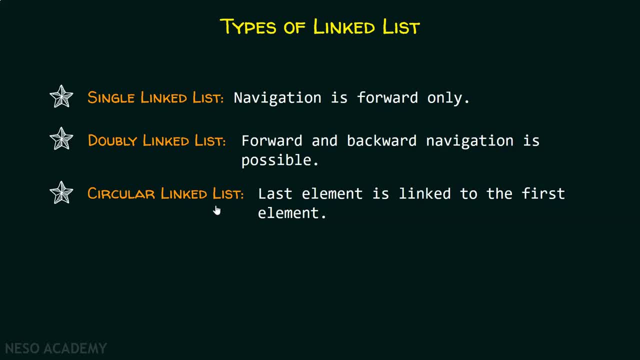 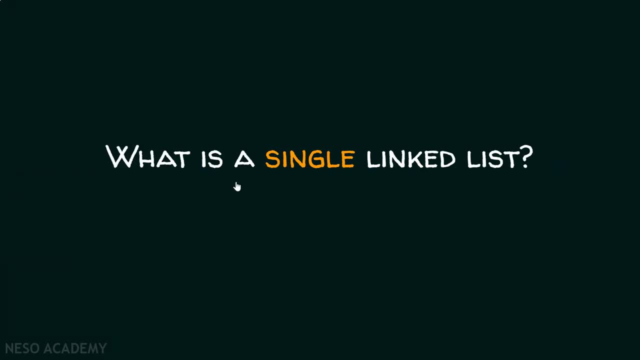 As the name itself suggests that this is a circular link list, So definitely the last element must be linked to the first element. Now we will discuss what is a single link list. A single link list is a list made up of nodes that consists of two parts. 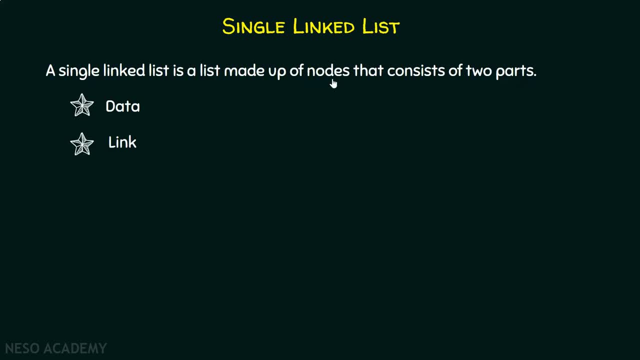 Basically, a single link list is a list made up of nodes. Now, what is a node? by the way, This is how a node looks like. This node contains two parts. The one is data and the other one is link. Data part contains the attributes: 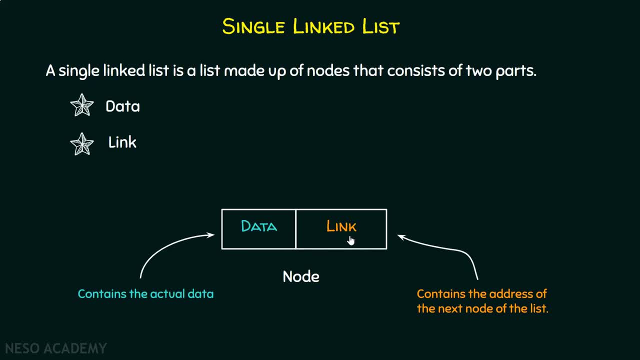 Actual data and link part contains the address of the next node of the list. If you ask me how a link list is made, I will simply give you this answer: that a link list is made up of nodes. Now we will see how to represent a single link list. 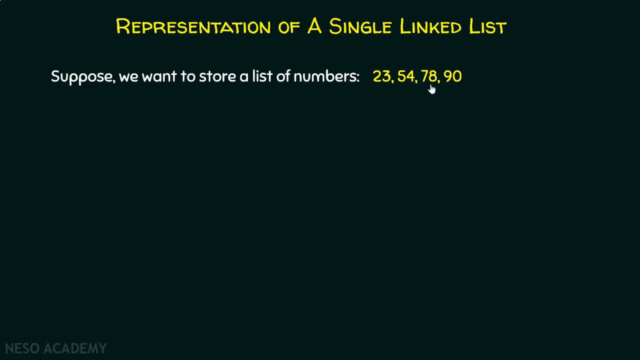 Suppose we want to store a list of numbers. These are the list of numbers we are available with: 23,, 54,, 78 and 90. For this purpose, I need to create four different nodes Because we have four different numbers to store. 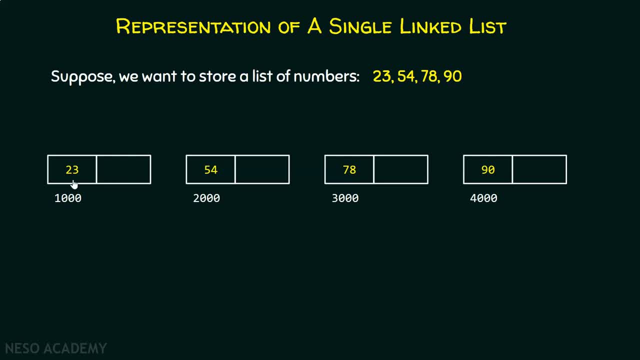 we need to create a list of four different nodes. The first node contains the data 23,. the second node contains the data 54,. third node contains the data 78 and fourth node contains the data 90. Now I would like to tell you that these nodes 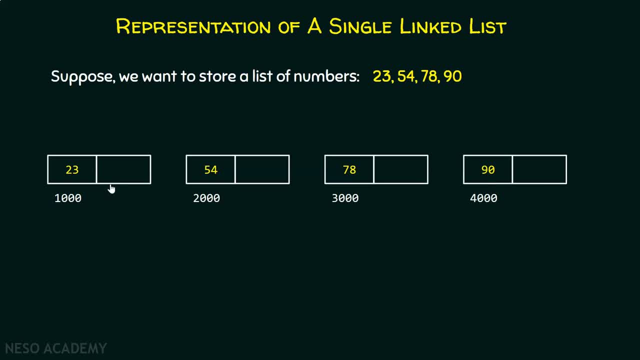 need not be stored in sequential order in memory. This should be well noted. For the simplicity sake, I have taken these addresses. The first node address is 1000,. second node address is 2000,. third node address is 3000. 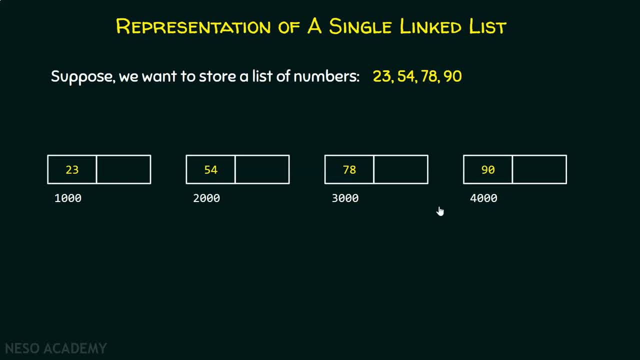 and fourth node address is 4000. And you can see. the addresses need not be sequential. This is not an array, this is a link list. Now, of course, there is something missing out here. This list is incomplete. Obviously, the list has not been created up to now. 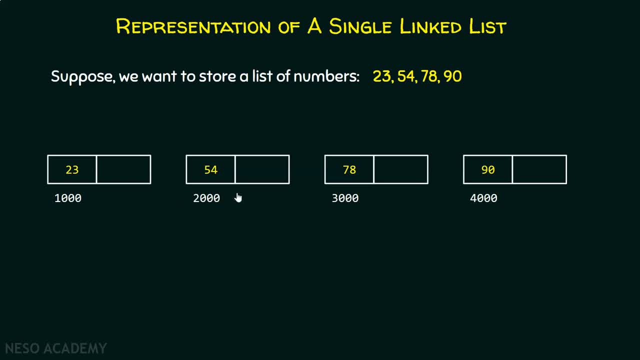 Because there is some way to reach the next node of the list And in order to do that, we will store the addresses in the link part of each and every node, How it looks like. Let's see. These are the addresses which we will store in the link part. 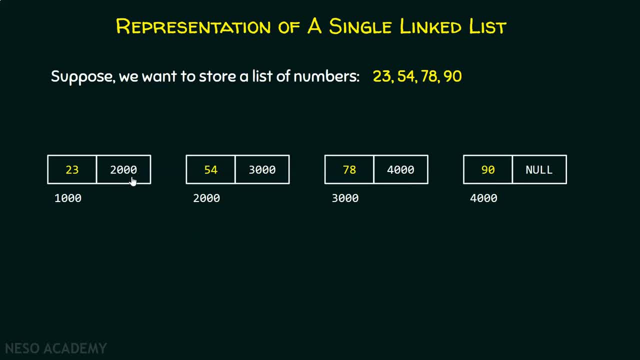 You can see that the first node contains this address, that is, 2000,. which is the address of the second node of the list, Isn't that so? From the first node I can easily reach the next node if I have this address. 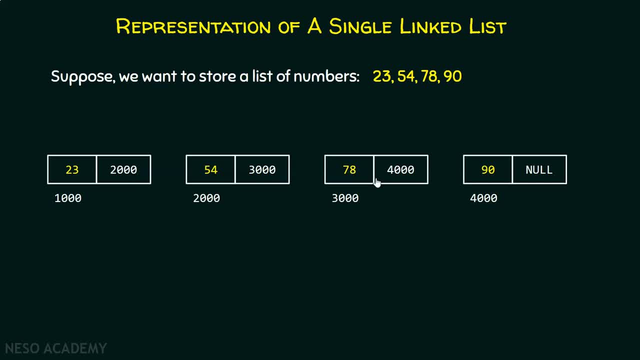 That is why I have stored this address over here. From the second node I can easily reach the third node because the address stored here is 3000, which is the address of the third node of the list, And third node contains the address 4000,. 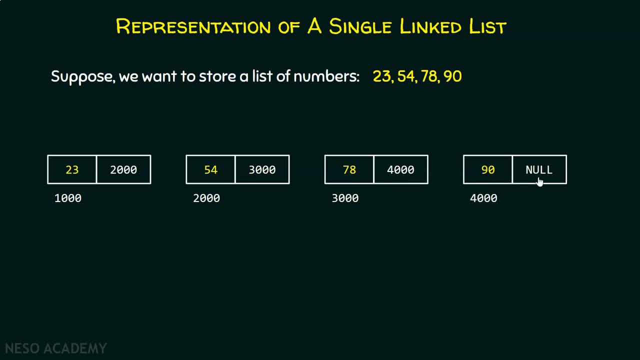 which is the address of the last node of the list. And last node contains null, which means it is not containing any address. It will simply not point to anything and it indicates that this is the last node Right. So basically, with the help of link, part of the node.